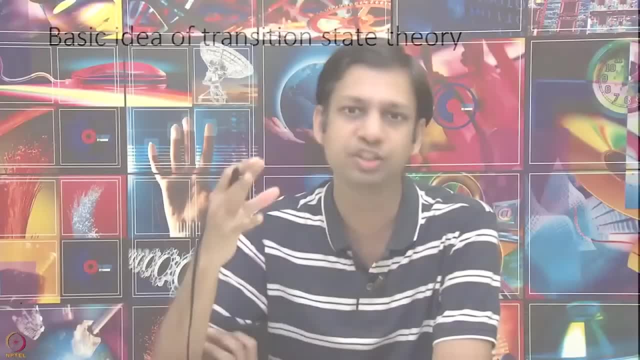 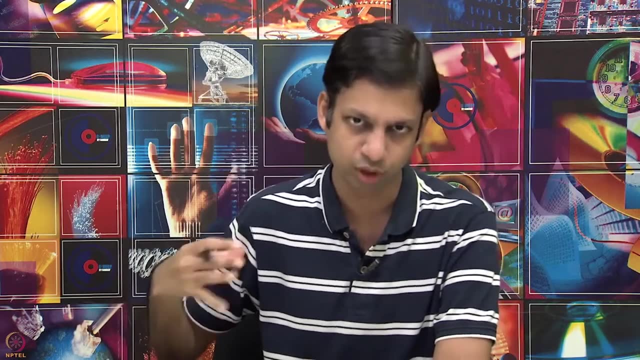 remembering kinetic theory of collisions. what is really missing is the idea of chemical bonding. The whole chemistry was missing, So we want to get that in into the picture. Okay, And we are in the, And we are essentially going to use the intuition that Arrhenius had provided. 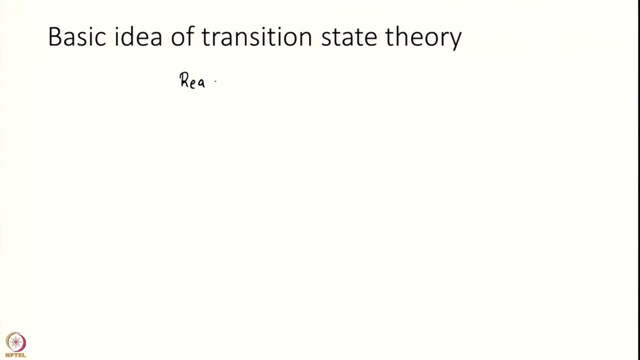 So let us start. let us say I have some reactants going to some products. the most general reaction reactants can be a combination or it can be bimolecular, unimolecular as any number of reactants to any number of products. So let me just write this in general, as R going to P, I do not mean this to be unimolecular. 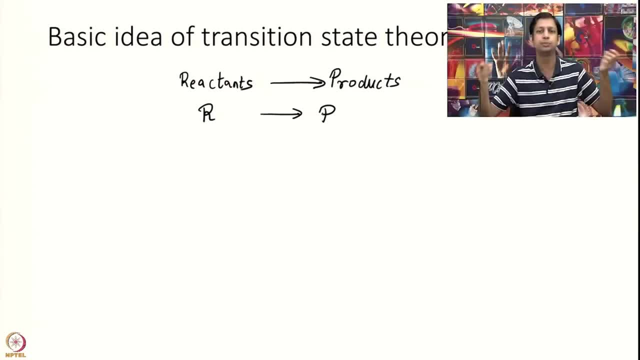 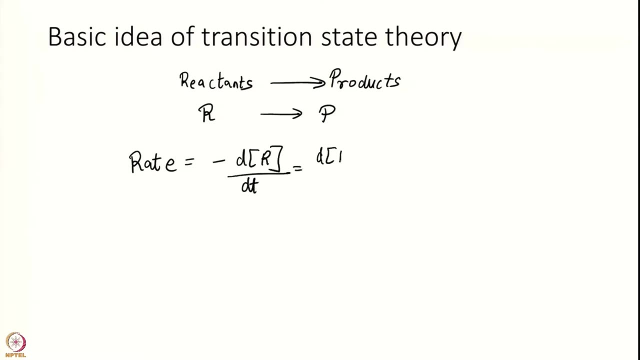 when I write R, R can be a plus b, R can be a plus b plus c, yeah some R, and eventually what we want to find is the rate which, if you remember, is defined to be this: at constant volume. Please do note that, in writing this definition of rate, I am not assuming this step is elementary. 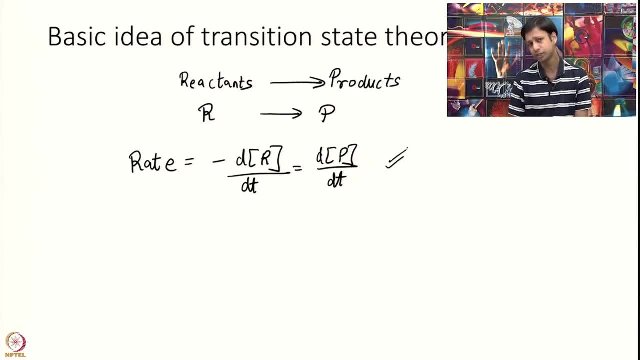 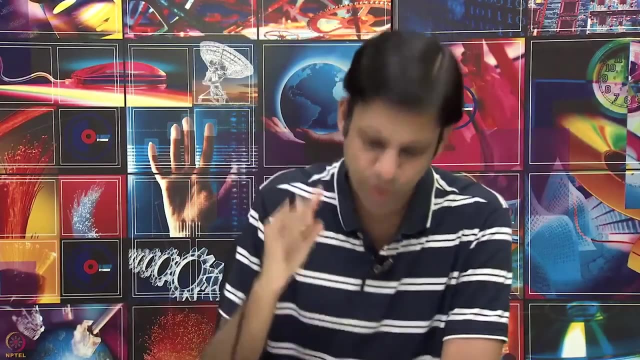 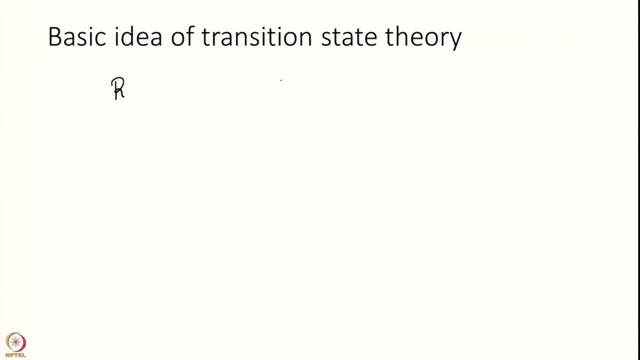 This equation holds as long as volume is constant. So this rate is what I want to find, and the postulate that transition state theory comes about is the following: I have these reactants and I have these products and we bring in the idea of transition state that Arrhenius was talking. 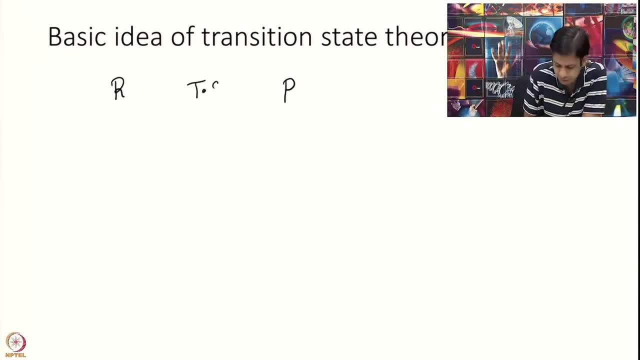 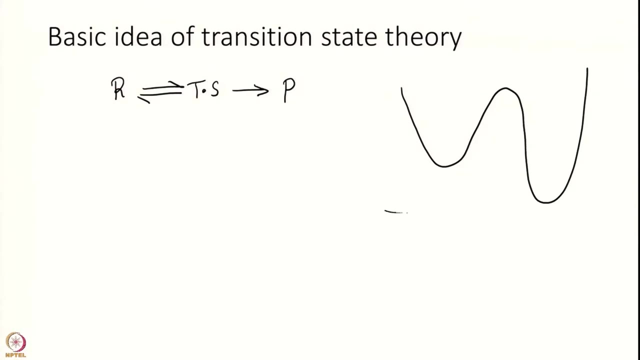 about Okay, And so I have a transition state in between and the reaction between reactant and transition state is one at equilibrium. So pictorially, the idea is: I have- I am drawing a 1D figure because that is easy to draw- I have. 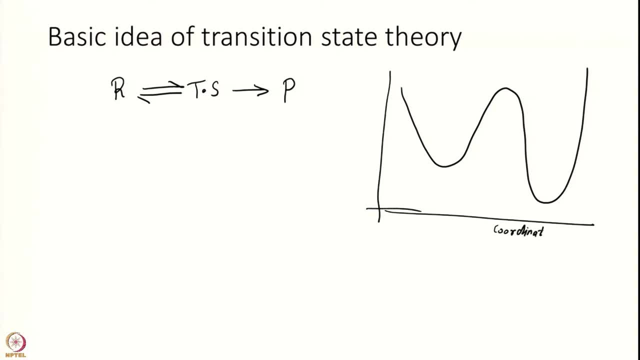 some coordinate here. call it the reaction coordinate, if you will. some potential energy here. So this is reactants, this is products and in between, since the transition state. So that is the main focus of transition state theory, the in between structure. So 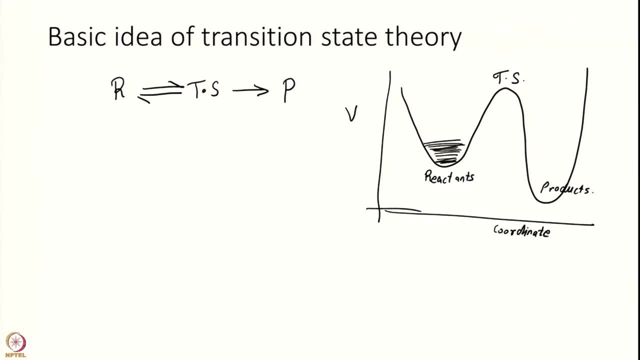 what we assume is that initially I am at reactants, So I am initially here and I have an equilibrium with transition state. I am at thermal equilibrium with the transition state, So reactants can go to to transition state, transition state can come back to reactants, But transition state can also. 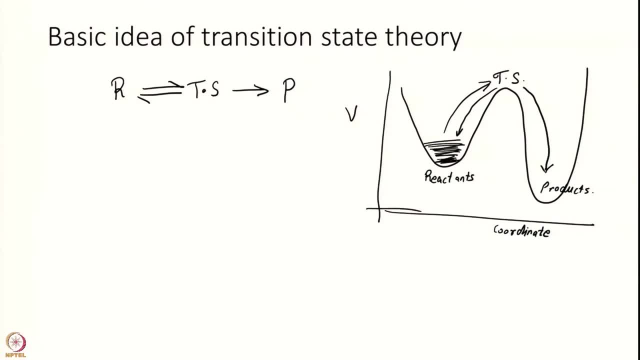 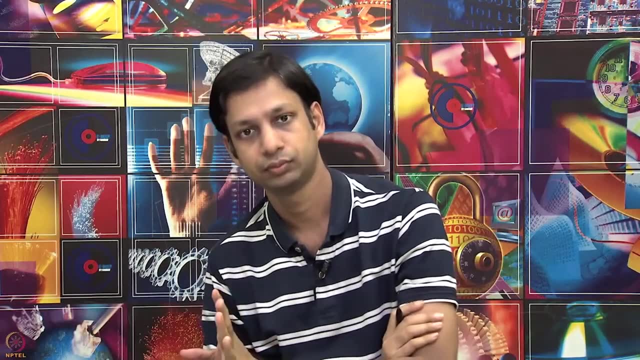 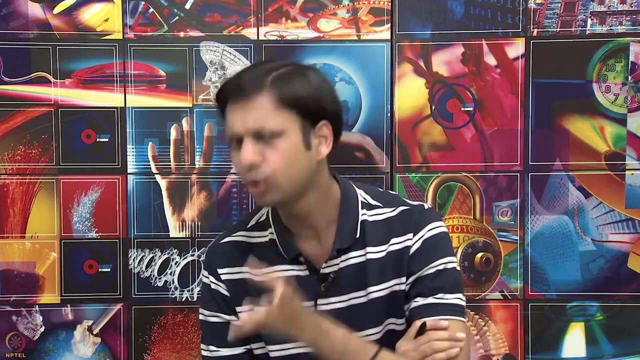 fall down to products And one of the critical assumptions of transition state is that going from transition state to product is one way. So there is no equilibrium, no back reaction from product to transition state. It is one of the critical assumptions and we are going to discuss. 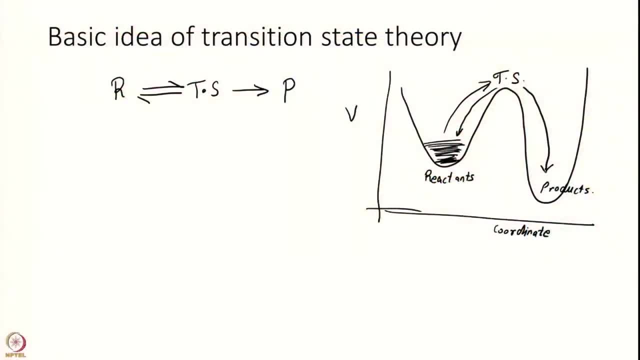 these assumptions in great detail later on. So let us think about this model. I have a k1 here and a k minus 1 here and I have some k2 here, and all these steps are assumed to be elementary. So if I want to find the rate rate was dp over dt, but I can look at this elementary step. 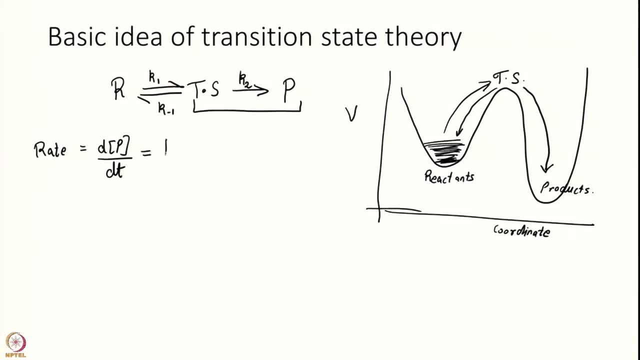 transition state going to product dp over dt will be equal to k2- into concentration of transition state. So that is how we write rate loss. You can go back to our very first module where we defined module 1 or module 2.. So the next thing we assume is that reactant and 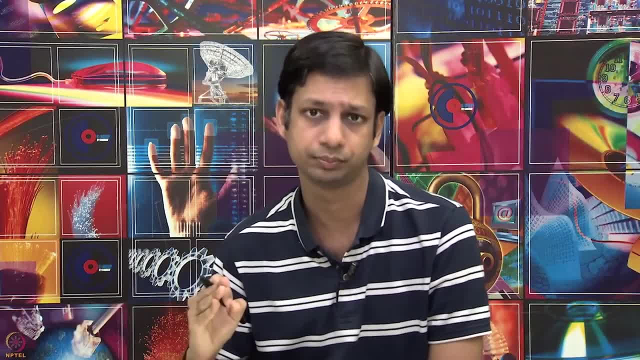 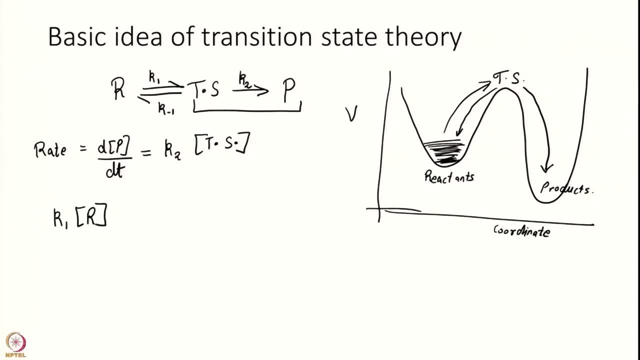 transition state are at thermal equilibrium, which means that the forward rate k1 into R, So this is R going to transition state. This rate is equal to the backwards rate, So this is forward rate k minus 1 into transition state, So this is the backward rate. 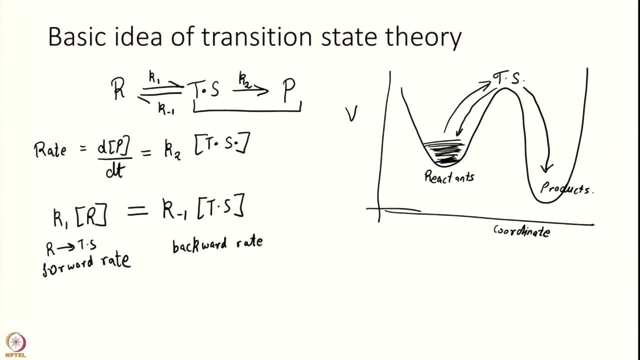 So at equilibrium, which is an assumption. So we are making some assumptions to build. our theory is equal to this. So from this I derive transition state concentration Equal to k1 over k minus 1 into R, and k1 over k minus 1 is what we call as k equilibrium. 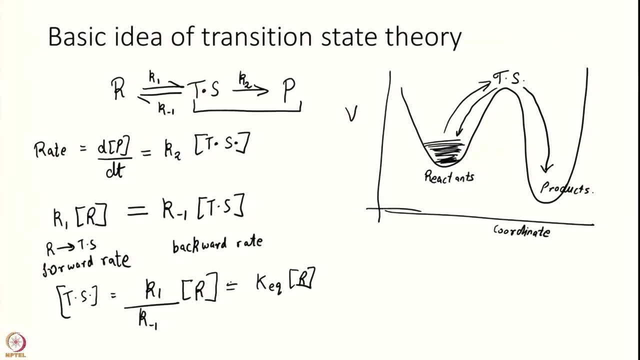 k equilibrium is the equilibrium constant of R with transition state, So my rate is then, so I use this equation here: k2 into concentration of transition state state, which we have found here. ok, And so the after doing this basic analysis making. 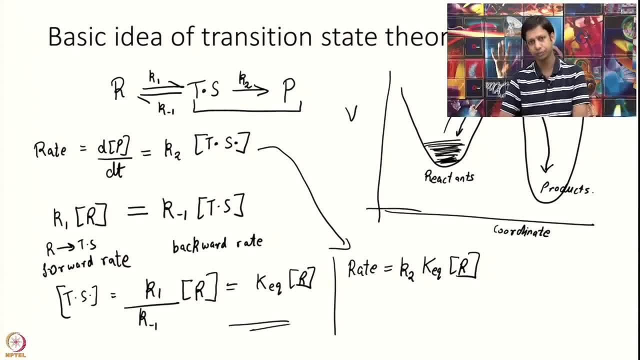 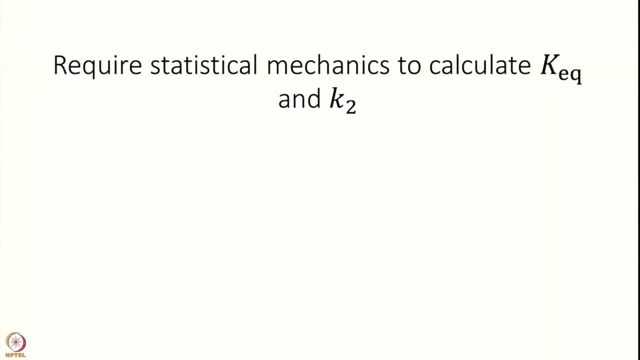 all these assumptions, what we have to do now is estimate k 2 and k equilibrium. ok, So to calculate this k equilibrium and k 2 we require a little bit of statistical mechanics. without that we cannot actually calculate this and, as it turns out, this k equilibrium. 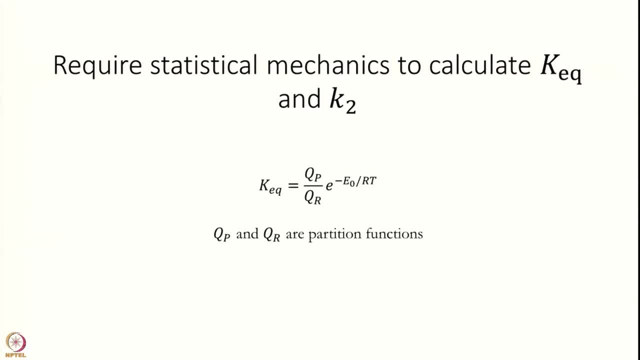 particularly is related to what is called partition functions. ok, So these relations are very fundamental in statistical mechanics and to understand these relations, we will need to study partition functions. all right, So that is what we are going to do in today's and next module, and perhaps the next one as well- is understanding. 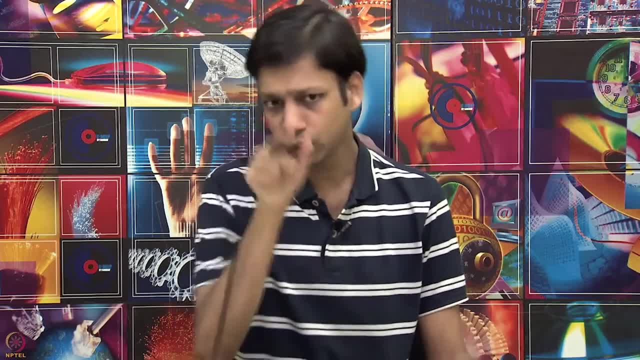 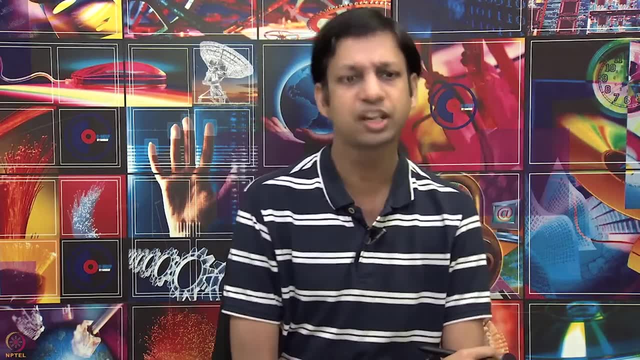 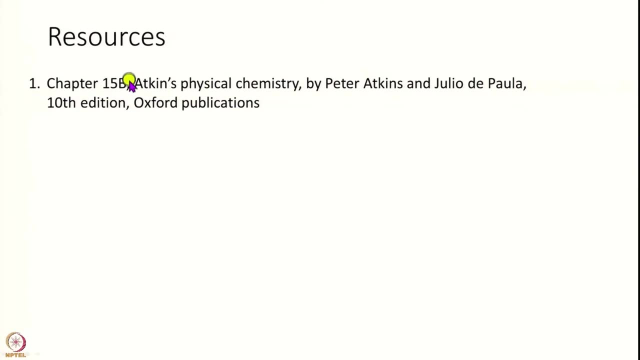 about capital understanding, then you need to learn about equalization, If the other partition functions, So that we can calculate this k equilibrium. ok, So this partition functions. you can read in the Atkins book: I have provided you this particular edition, 10th edition, chapter 15b. You have any other edition? please do not worry, you will be able. 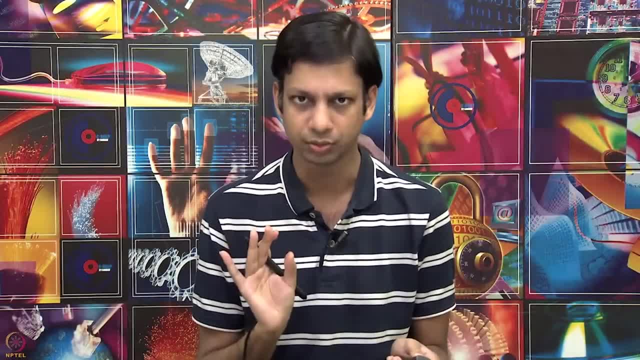 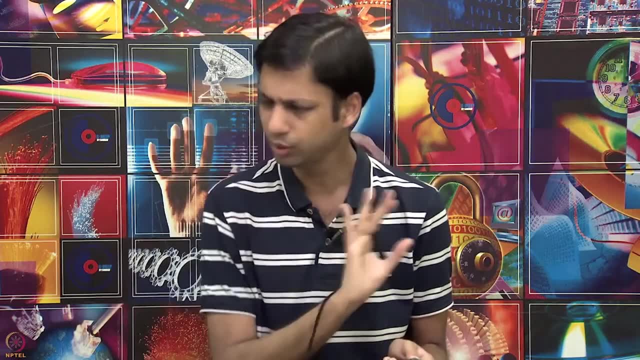 to find this particular content in some other chapter number. The content remains the same in the chapter number changes, So you do not have to spend more money in getting the 10th edition. ok, You will be able to find it in any other edition, Of course. partition. 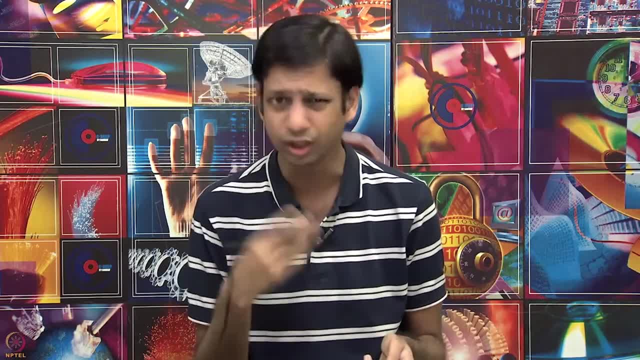 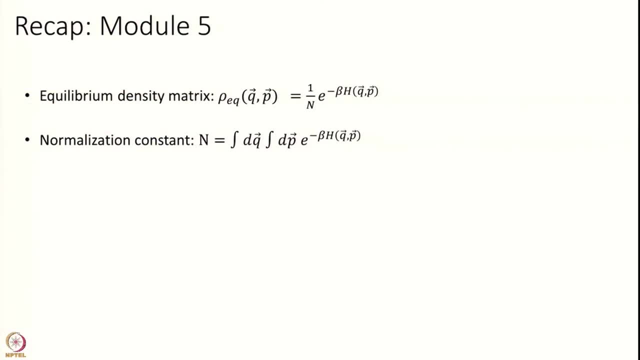 functions you can find in many other standard textbooks of statistical mechanics or even online. ok, So we will recap something very old, Much ago, 10 modules ago, we derived something very fundamental: that at equilibrium the classical density matrix looks like 1 over n into e to the power of minus beta h. 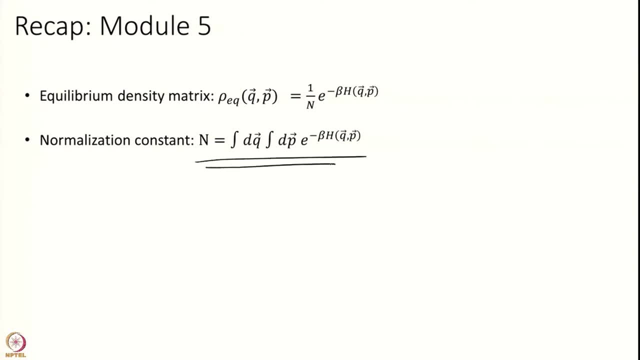 And my n, which is a normalization constant we showed is equal to this. You can go back to this module where we did partial derivation in phase space. We will build over it right now. So the point is, first thing, we note: what is the units of n? Well, it is, we see. 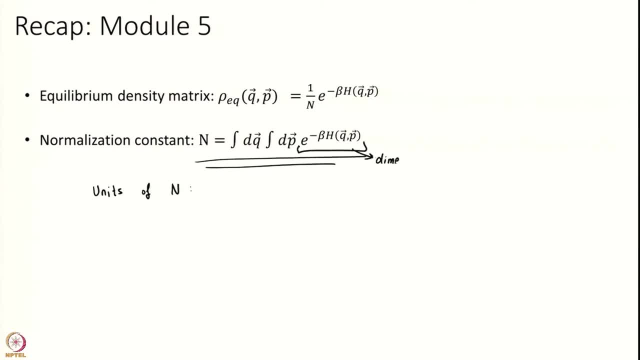 that this thing is dimensionless. it is an exponential. So the units of n is the same unit as q into p. ok, What is the dimension of 1 q into 1 p That is equal to q is unit of length, So in SI units it is meter. p is momentum, which is kilogram meter per second. 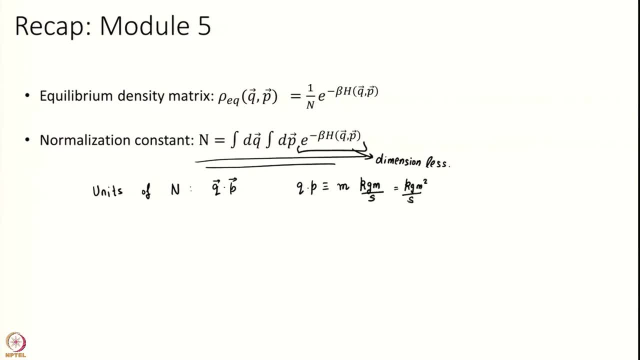 which is kilogram meter square per second. Does this unit remind you of any fundamental constant of nature? It should strike you something that is related to kilogram meter per square per second. If you guessed h or h bar, you are exactly right. This is the same units. 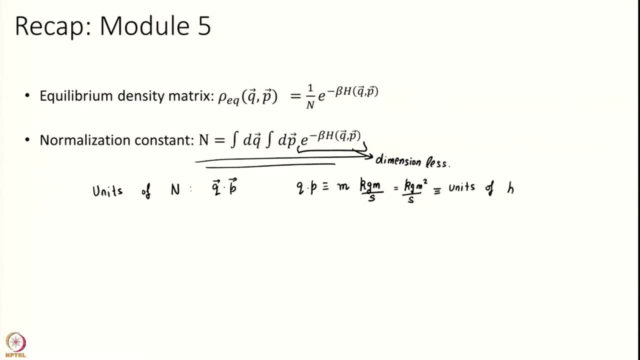 of h, the Planck's constant. ok, So q dot p, this is 3.5.. 3 n q dot p. So q is a 3 n dimensional vector, where n is the number of particles. So this: 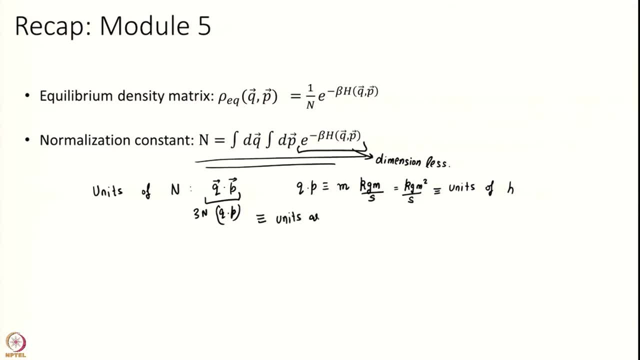 thing is the same units as h to the power of 3 n. Each q dot p gives me 1 h. I have 3 n q dot p, So I get h to the power of 3 n. So the first thing we do actually is to: 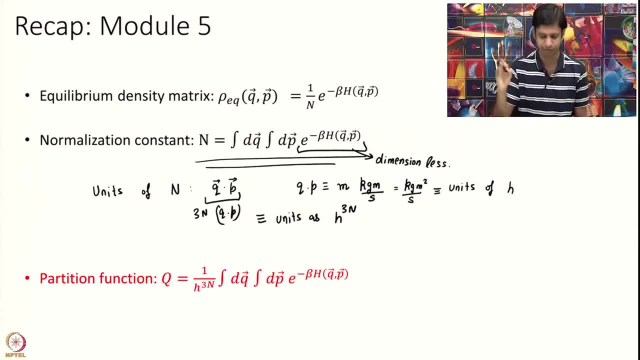 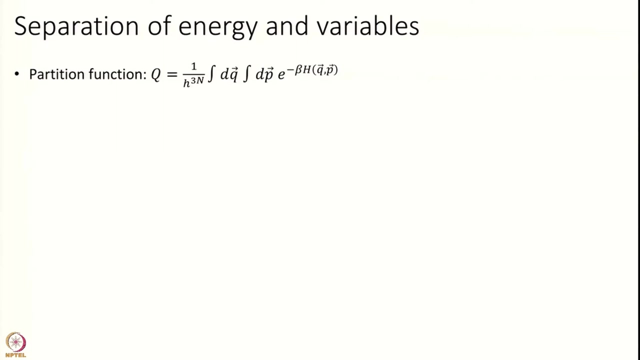 define a partition function, q, which is dimensionless. So we take this n and divide by h to the power of 3, n. So this thing is dimensionless. So we start with this partition function and what we do is This by itself is very large, very, very complex to calculate. This is a 3,, 6 n dimensional. 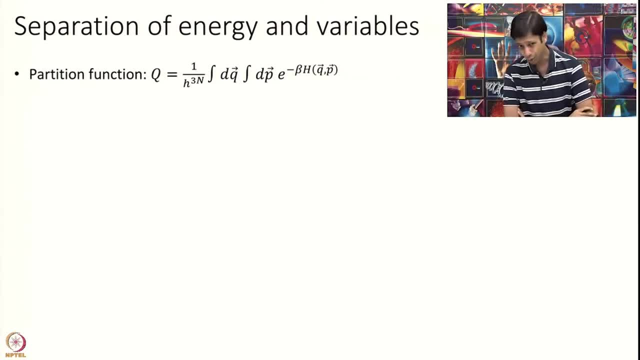 integral. I have 3 n q's. I have 3 n p's. I do not want to do this integral. I do not know how to do this integral. We will simplify our life. What we do is we note one important. 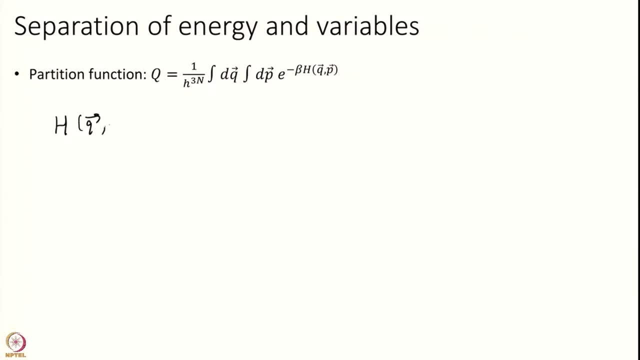 property of the Hamiltonian. This to a good approximation, for most problems can be separated into Hamiltonian of translation plus Hamiltonian of rotation plus Hamiltonian of vibration. once we bring in quantum mechanics we will also have an electronic part. but that I am. 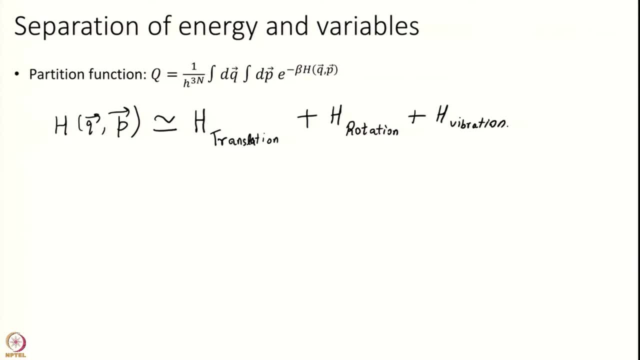 not writing right now, So this is an approximation. This is not always separable. This may be to Translational part can always be separated, but rotation and vibration in principle can be mixed. but we will make this simplification for now, for this course, ok. 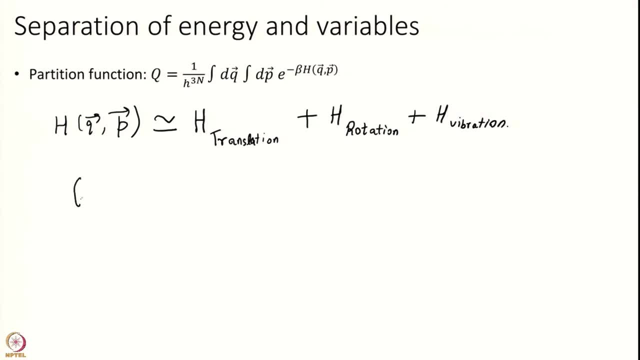 How do we make this simplification? Let us. we will have to provide one more thing, the q comma p, these are 6 n variables. This itself is partitioned into translational, which is nothing but center of mass. So these are 3 coordinates, 3 into 2, 6 variables, so the entire center of mass of the my molecule. 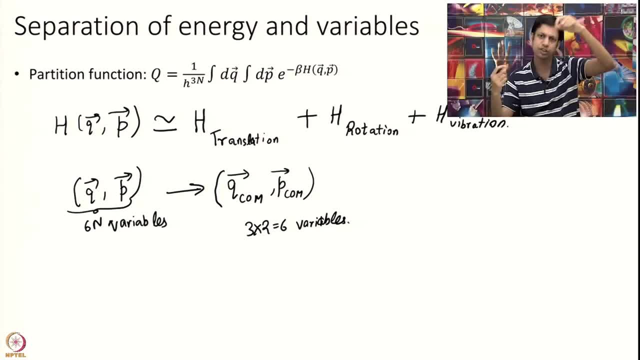 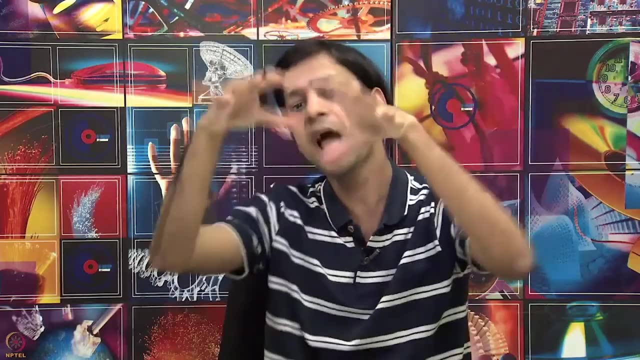 ok. So x, y, z of center of mass and p, x, p, y, p z of my center of mass. ok. Plus I have also coordinates and momenta describing rotation, So that tells me how the molecule is oriented and what is the angular momentum of my molecule. 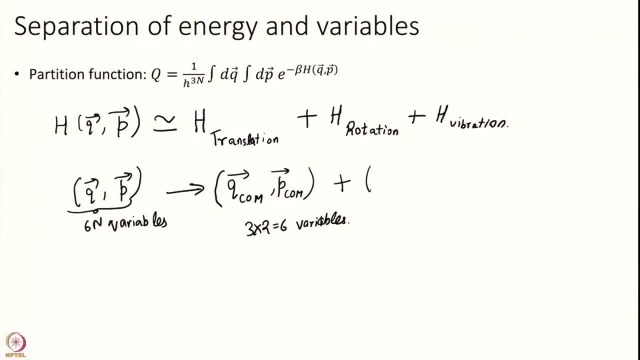 of the overall molecule. ok, how it is rotating around. So I have q rotation, comma p rotation. so this is a slightly more complex. for linear molecule There are only 2 rotations possible. we will discuss this in a moment. so 2 into 2, 2 angles. 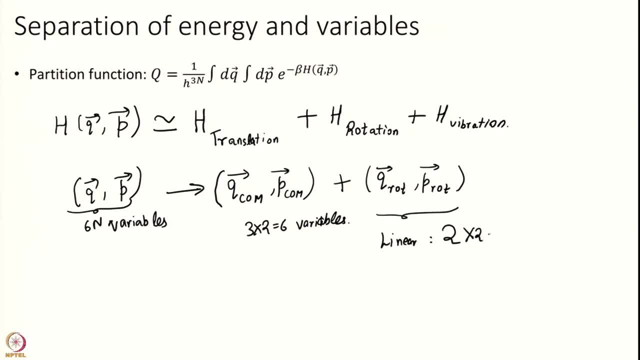 and 2 corresponding angular momenta, so 4 variables For non-linear. we will discuss this in the next slide. please do not worry. we can have 3 possible rotations. We have q comma, p of vibrations. ok, so not only do we separate out the Hamiltonian, we 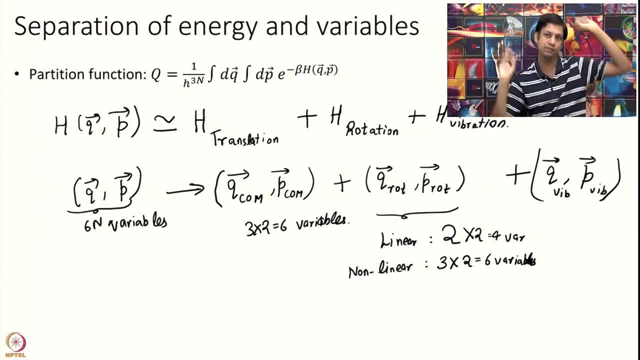 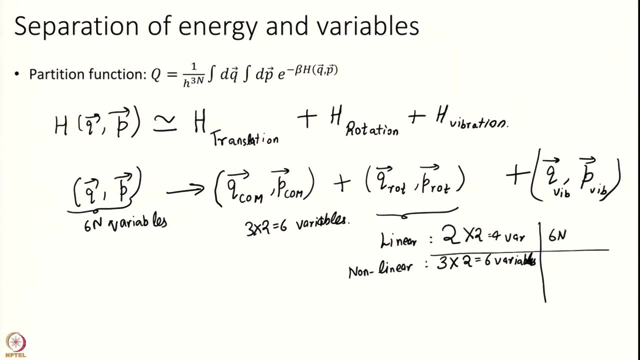 have also separated outer coordinates and momenta. We have coordinates describing translation, coordinates describing rotation and coordinates describing vibrations. So again, for linear you vibrations will essentially become 6 n minus 4.. Remember the total has to be 6 n. I had 6 n variables here. I should have 6 n variables. 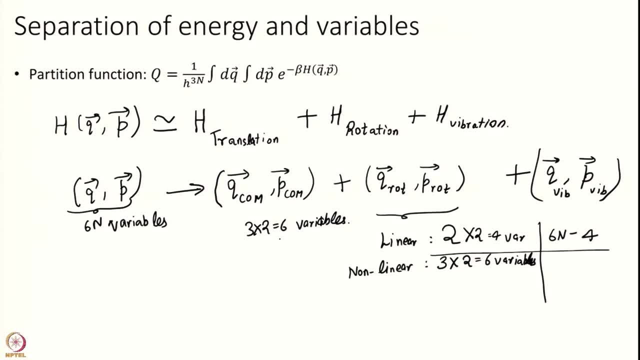 on the right. 6 have been taken for translation, 4 for rotation, so I am sorry. my maths should become 6: n minus 10. for linear and for non-linear this will become 6 n minus 6 plus 6 is 10,. 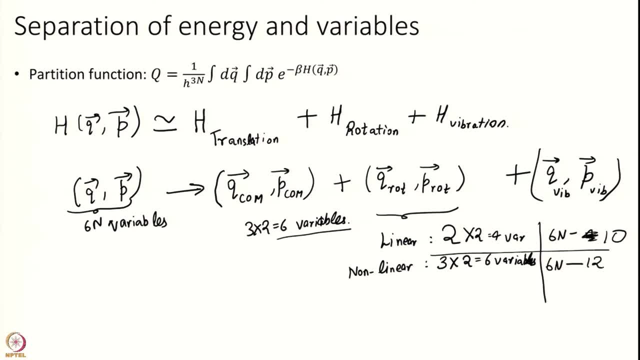 12 minus 12.. So I will have 6 n minus 10 vibrations, vibrational degrees of freedom for linear molecules and 6 n minus 12 for non-linear. So let us look at an example. things will become clearer. 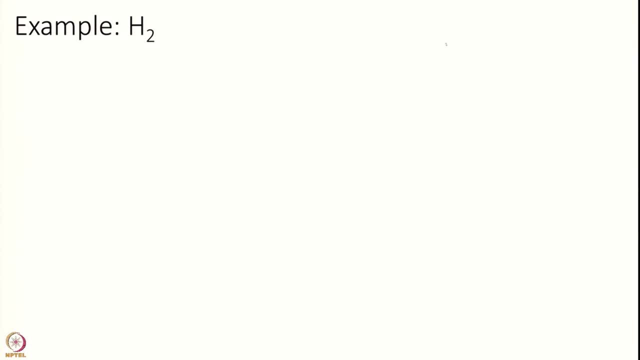 So let us start with a very simple linear molecule, H2,. so let me just draw x, y, z and let us say I have some H2 molecule oriented somewhere here. So I have x 1, y 1, z 1 of the first and x 2, y 2 and z 2 of the second. hydrogen. 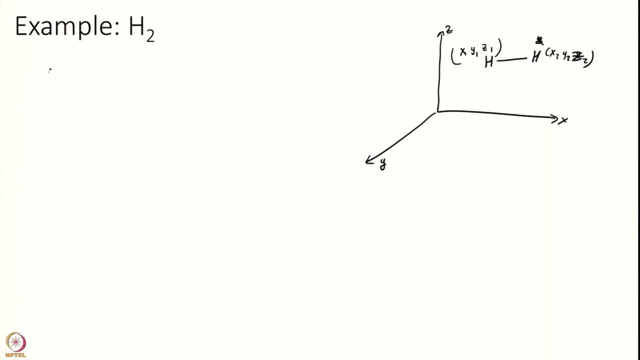 So I have a 6 coordinates, which is basically x 1, y 1, z 1, x 2, y 2, z 2, and we transform this into a 3. into 3, center of mass. So we find a center of mass here. 3 center of mass coordinates. 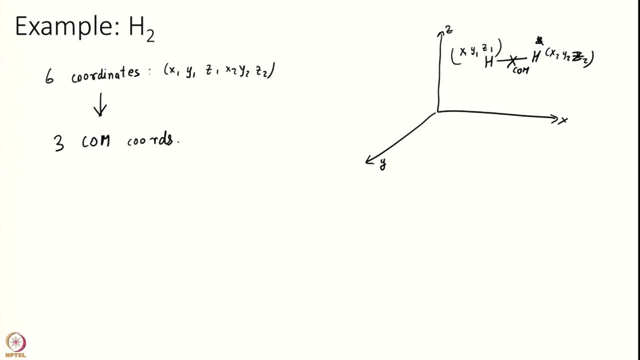 Now this molecule can rotate in 2 ways. One is this rotation in plane: 1 in plane rotation plus 1 out of plane rotation. So for this molecule I have to tell you theta and phi. essentially is what I am saying: You give me center of mass and you give me how the 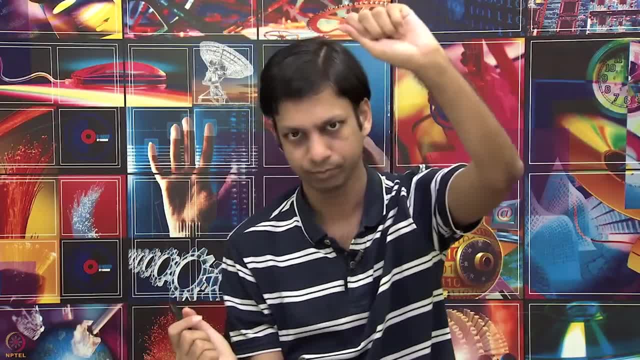 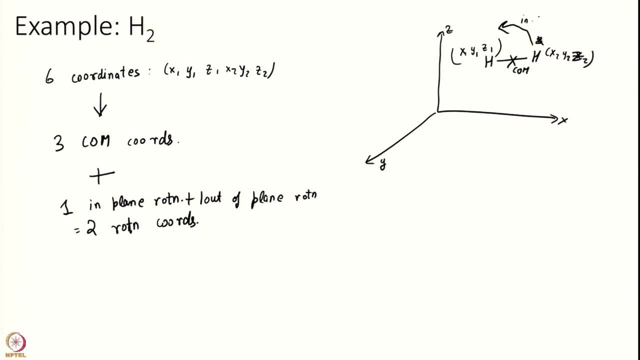 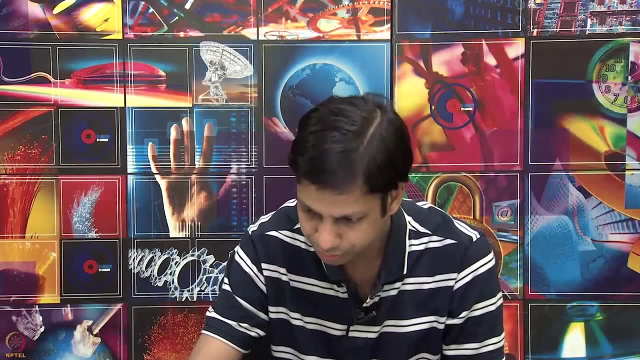 molecule is oriented in space, which can be described by theta and phi right. So for a linear molecule Only 2 are enough. So one is in plane rotation and the other is. imagine this h 2 coming out of plane like this. So it is a hard thing to draw, but you can imagine something like: 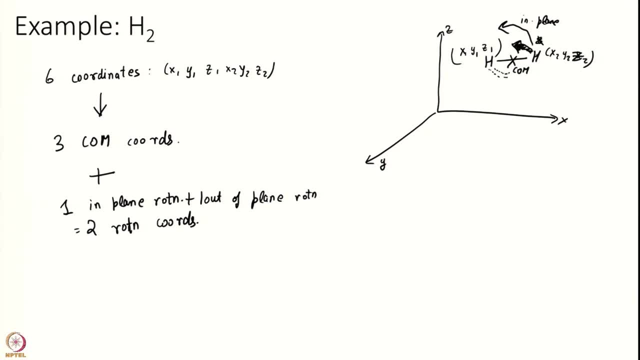 this and this h is going under the plane, something like this. So the whole thing is rotating around like this. ok, And plus I have 1 vibration, h. 2 can have only 1 vibration, which is which is this length. let me call this x. So you see, I have a total of 6, 3. center of mass. 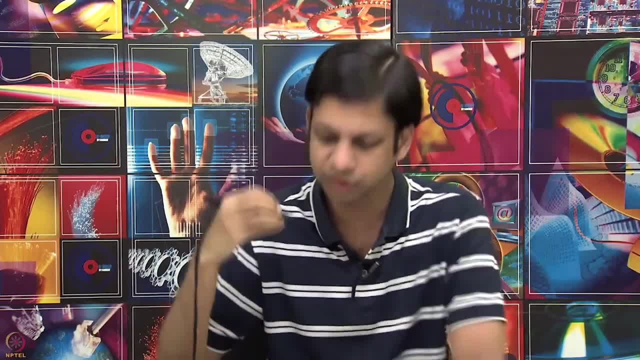 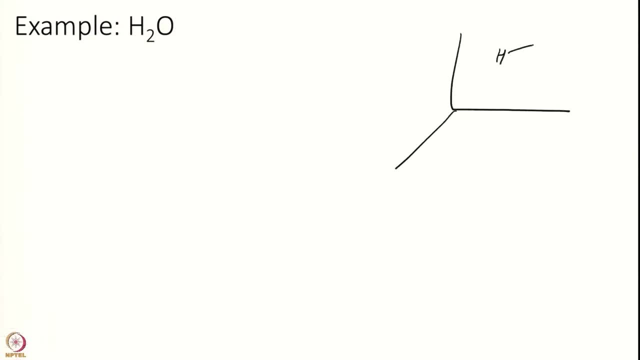 2 rotation 1- vibration. Let us look at a slightly more complex example which is non-linear. Let us look at water, So I have some orientation of water sitting here. Again, I have x, y, z, So now I have 9 total coordinates: x 1, x 2,, x 3, x 4, x 5,, x 6, x 7, x 8,, x 9,, x 10,. 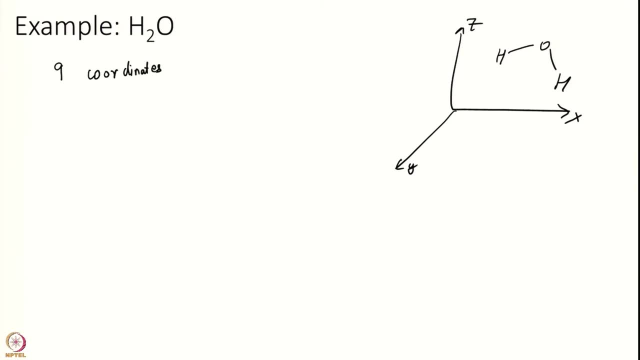 x 11, y 1, z 1 of hydrogen: x 1, y 1, z 1 of the second hydrogen: x 2, x 3, y 3, z 3 of the oxygen. So again, I will always get 3 center of mass. So wherever the center of mass lies, Plus, 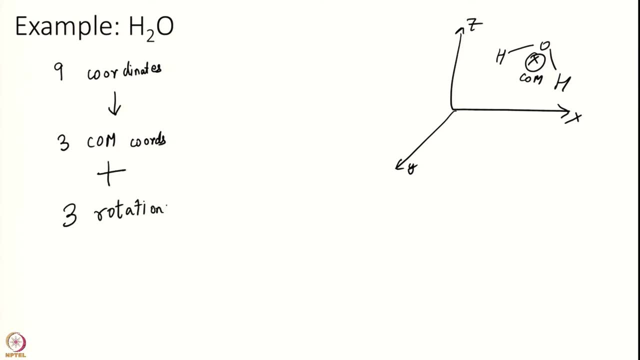 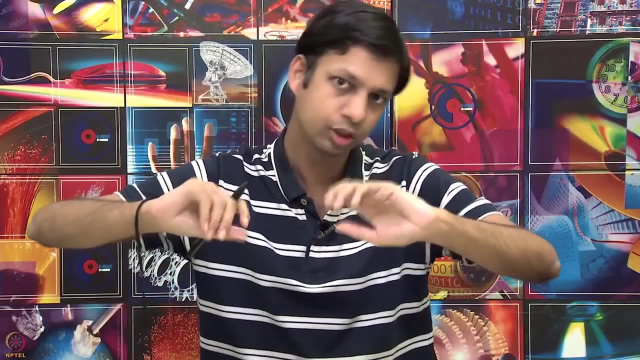 this time I will have 3 rotations. Why? Because you also have to describe how the water it itself is oriented. So theta and phi tells me the overall structure, but beyond that as well, the molecule has internal structure. So I can have a one more degree of freedom. 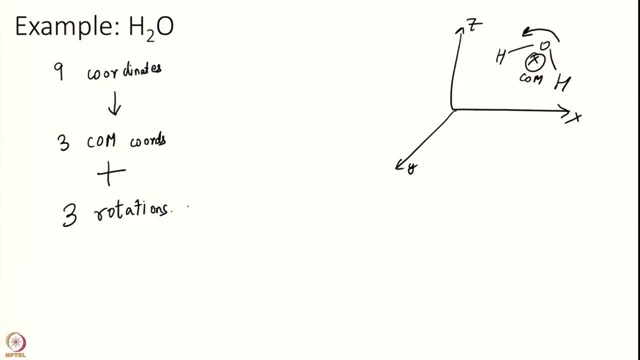 More physically. essentially you have 1 in in, 1 in plane and 2 out of plane, So I can rotate the whole molecule in that direction. Next slide: this manner. but I can also rotate the whole molecule in this manner. So one is in the 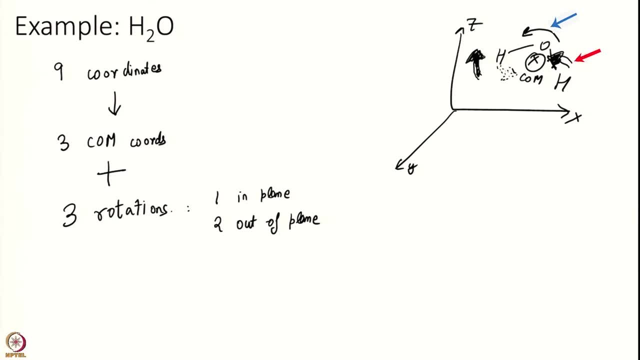 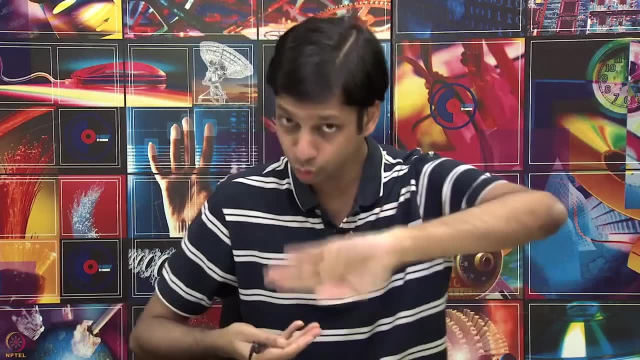 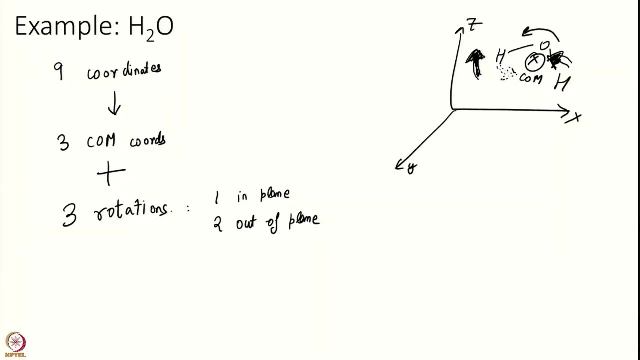 plane. one is out of the plane like this and I can also rotate it like this for three possible rotations For H2, this was not possible because your H2 is rotating around the one axis. It is yeah, so it that does not rotate at all. So that is the issue and I have three vibrations. 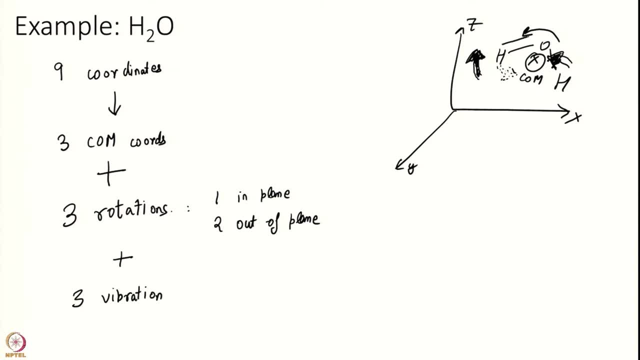 So for water, I can have this stretch x1, I have this stretch x2 and finally I have the angle theta. ok, So I have three vibrations possible. So the match will always work out. ok, So we have separated the energy. Let me just tell you a little bit more. So the translational 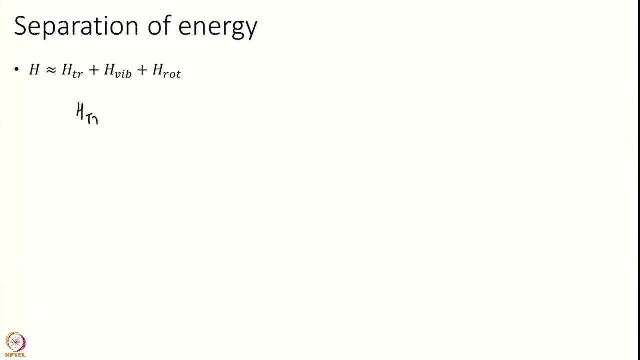 energy is essentially that of center of mass. ok, So this basically looks like momentum of center of mass, square divided by 2 m, where m is the sum of all masses. So m is the sum of all atoms, sum of- sorry masses of all atoms. ok. 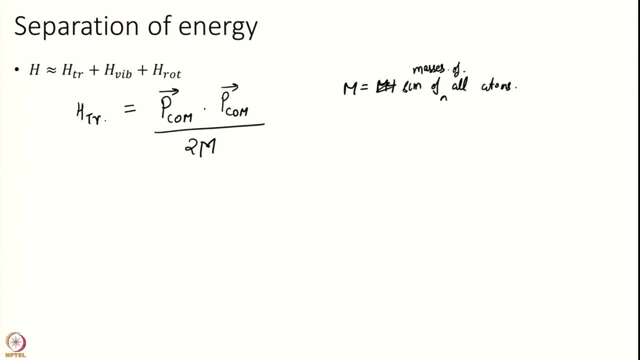 So that is your translational energy. Just the kinetic energy of your center of mass Rotation gets a little bit more complex. So I will not write the complex descriptions here, which is not necessary for this course. This essentially is the angular momentum. 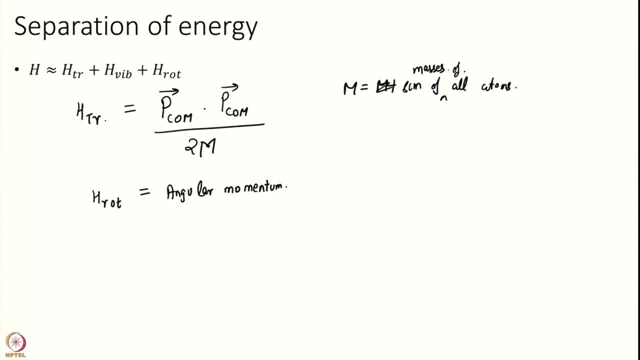 which is like l square over m square. So they have these transformations and I am not simply like L square over 2 I. and finally, is the vibration which essentially looks like harmonic oscillators. ok, So you have something like p square over 2 mu plus half mu r square, something. 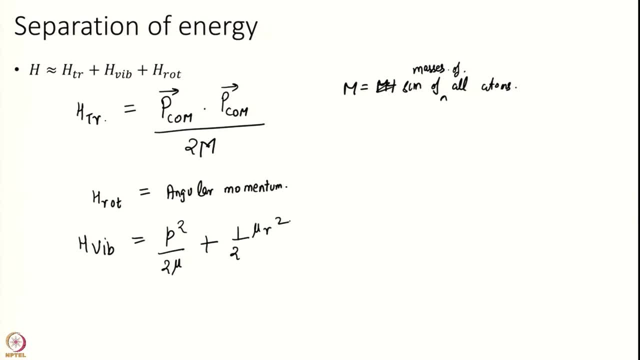 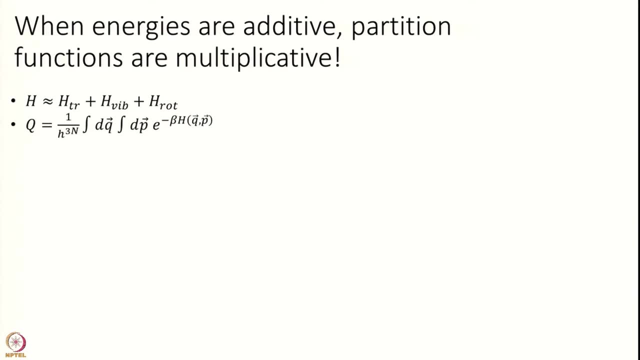 like that. ok, where r is your vibrational degree of freedom? ok, So we have this separation of Hamiltonian. whatever the Hamiltonians are, let us not getting to one the Hamiltonian I right away. But let us look at this structure and let us put. 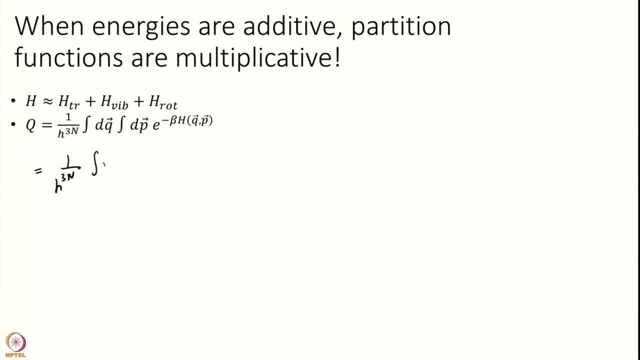 the separation of variable and the separation of Hamiltonian here. So remember, my q and p are now separated out. So I will write integral of dq, dp In terms of q and p, of rotational- sorry- and vibrational, and Hamiltonian also I am separating out. 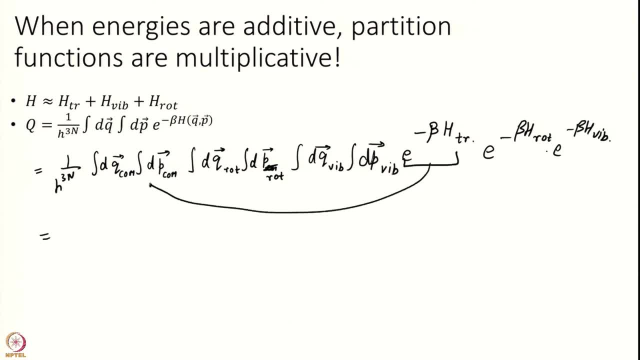 And then what we do is we? this depends only on center of mass, and this depends on this, and this depends on this. So I can write this as 1 over h cube, dq. center of mass, dp, center of mass e to the power of minus beta h translation. 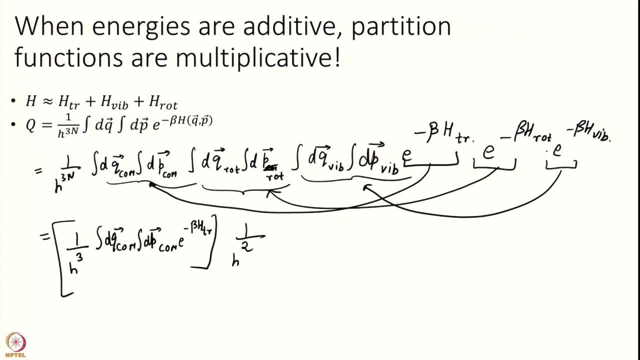 1 over h square for linear and h cube for non-linear. you understand that now it does not matter. and finally, vibrations. And depending on linear or non-linear, I will have 1 over h to the power of minus beta, h to the power of 6 n minus 5, sorry, 3 n minus 5 or 3 n minus 6.. 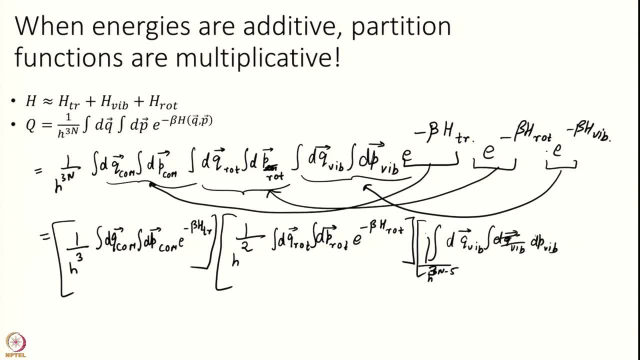 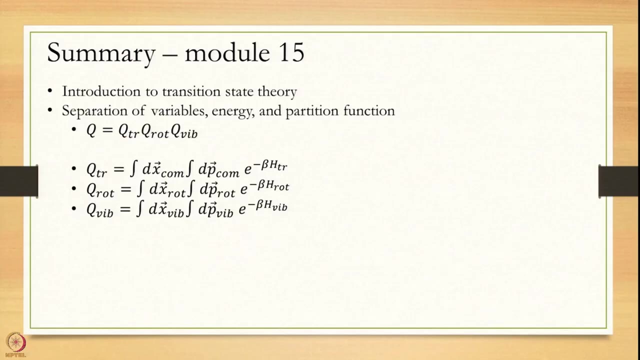 This should be dpy. so we call this one Q translational. we call this one Q rotation, whatever it is, h cube or h square, Okay, Okay, Okay, Okay, Okay, Okay, Okay. And this one we call Q vibration.